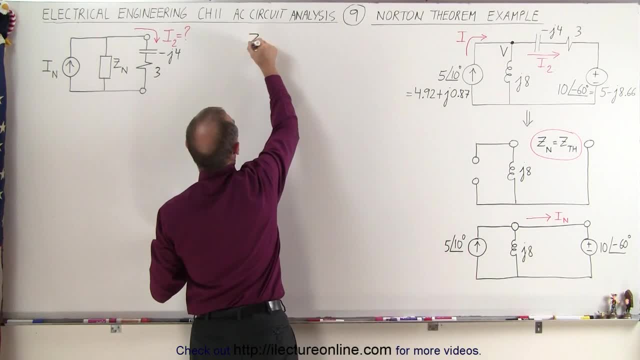 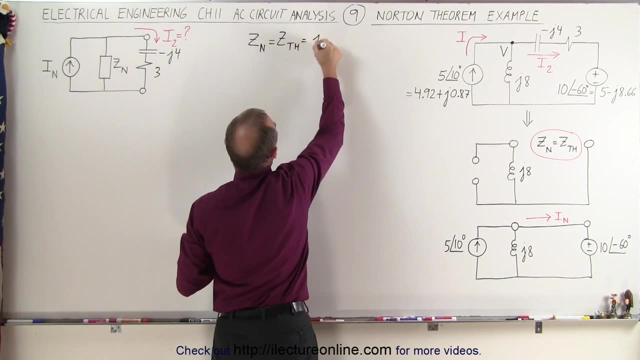 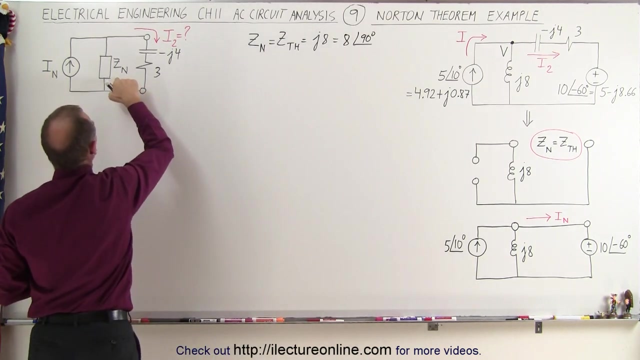 inductor right here. So it means we can write that Z Norton, the impedance Norton, is equal to the impedance Thevenin, which in this case is j8, which is equal to 8, with a phase angle of 90 degrees, which is what goes right here, so this becomes equal to j8.. The next thing we need to do is find: 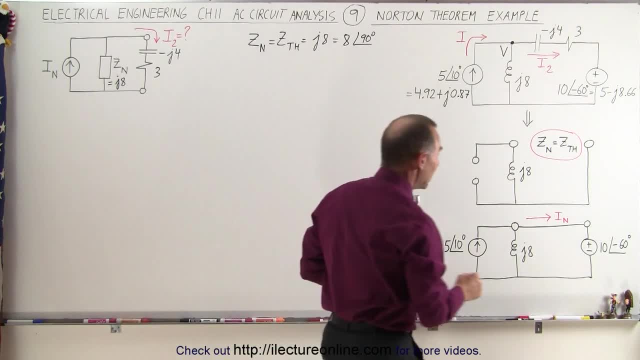 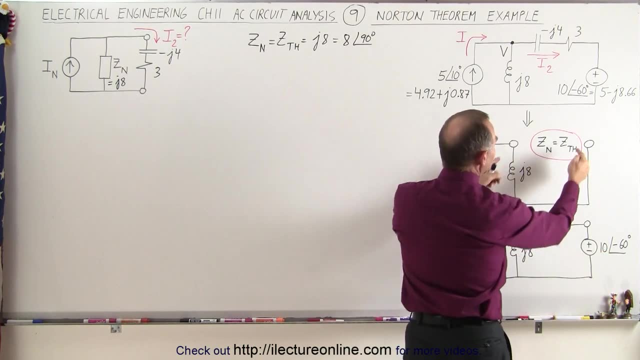 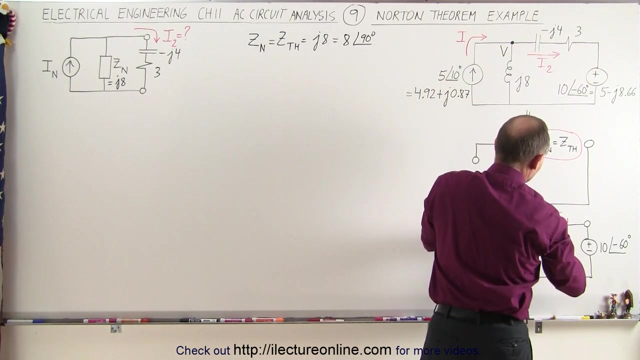 the Norton current, To find the Norton current. what we need to do, then, is we we have to put back our source current. we put back our source voltage and we take the, the load- in this case the load impedance- of the capacitor and the resistor and replace it by a short, and now we're trying to 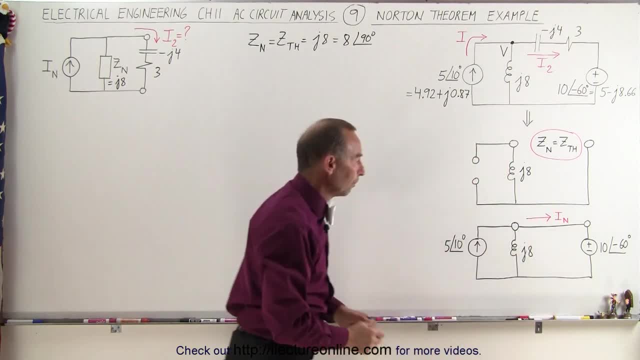 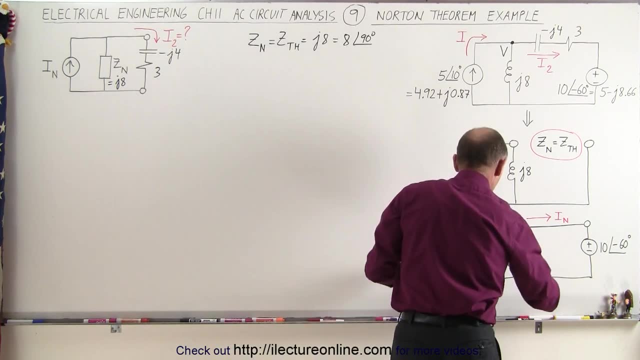 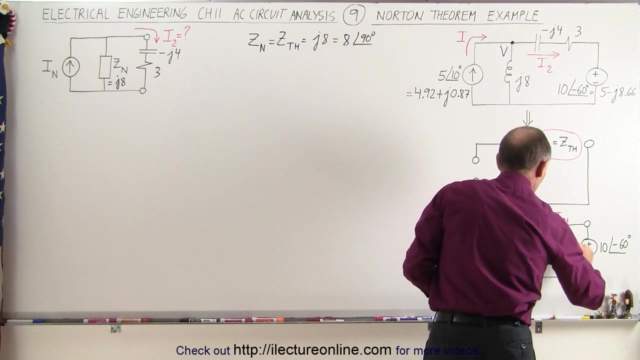 find the been into that short. that will then be the Norton current. How do we do that? Well, in this case we have to kind of use this method right here. So let's call this, call it current a, so I sub A, and let's call this current, I sub e, and then we use kind of what we would call. 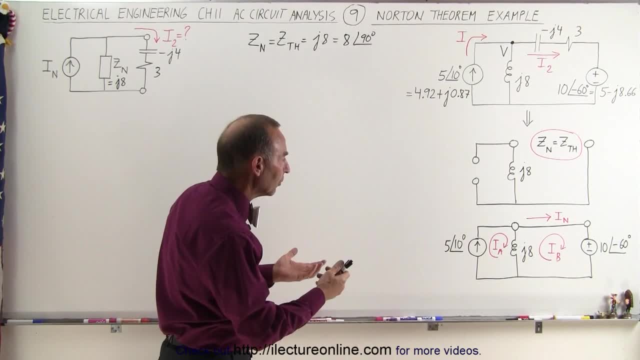 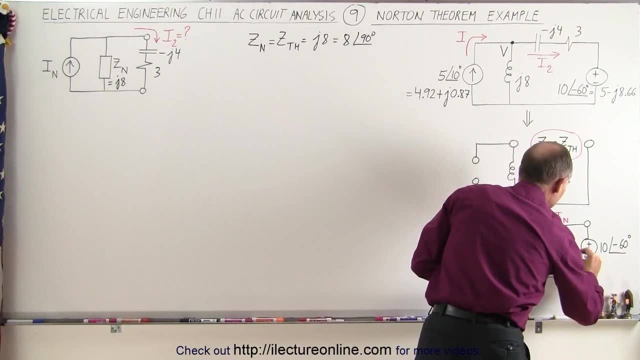 the nodal method, uh, to find the current through I sub n, which in this example here is an mm North to a short case, will be i sub b. so i sub b will be equal to i sub n, and so we're going to solve for those. 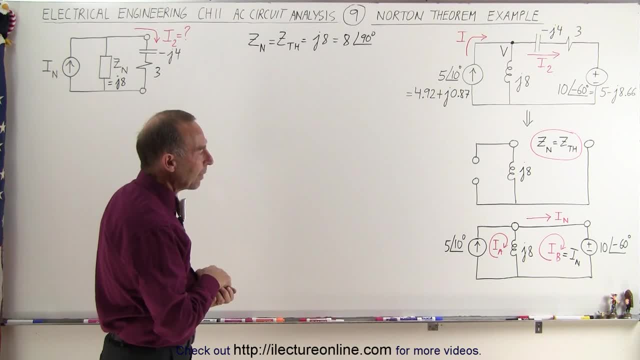 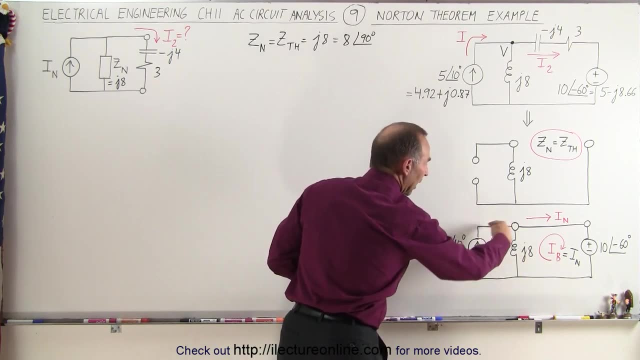 circuits right there, what we probably could do. well, now i'm going to show you the entire way of doing this. so first, let's go ahead and sum up all the voltages around this mesh right here. so let's let's call this the mesh, the mesh method. we're going to add up all the voltage around. 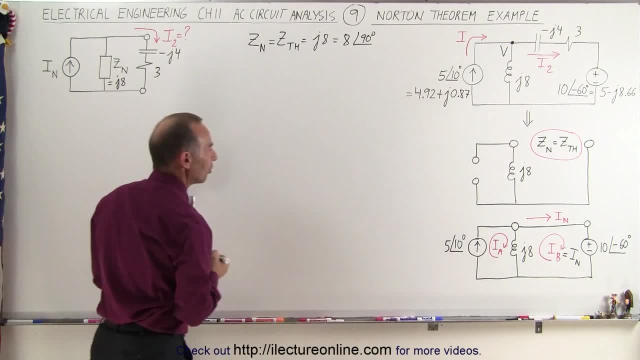 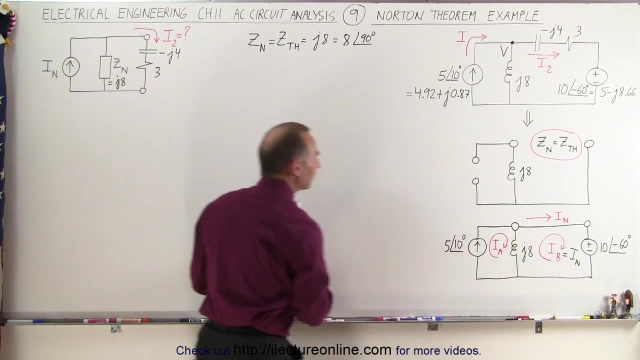 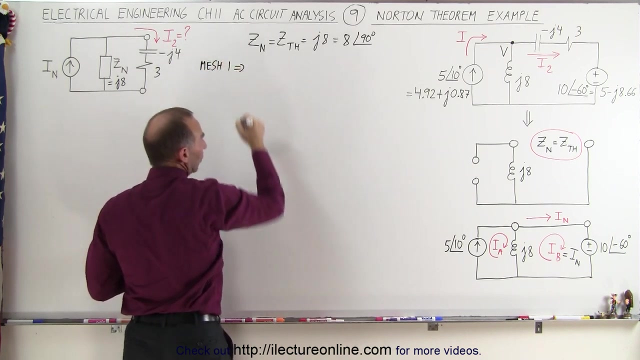 this mesh and we're going to add up all the voltages around that mesh, so no voltage drop across the current source, but we do have a voltage drop across the inductor. since we're going this direction, we can then say that for the first loop or for mesh one, for mesh one we have 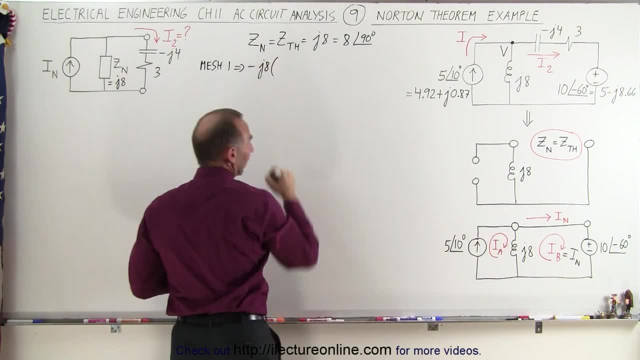 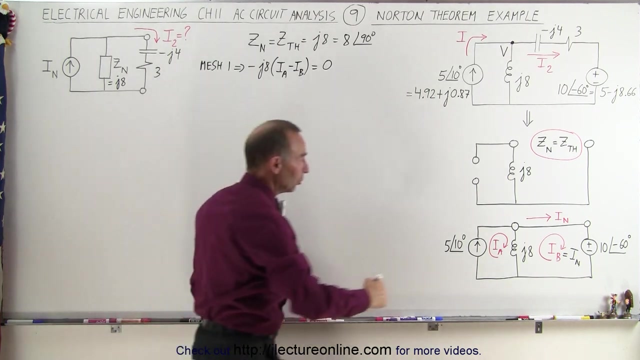 minus j8, multiplied times ia minus ib, because ib is in the opposite direction. so it would be ia minus ib, and since we then come all the way around the loop, that should equal zero. around the second mesh we do the same thing. let's start from here, go all the way around. 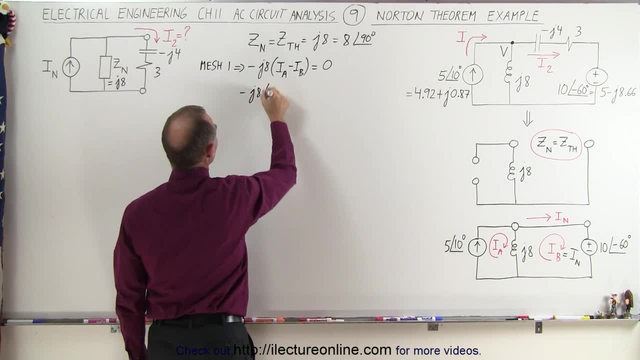 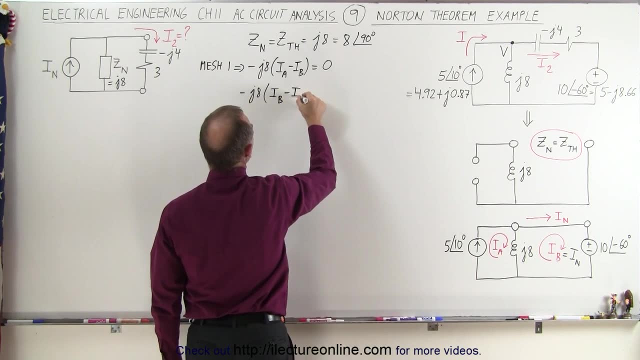 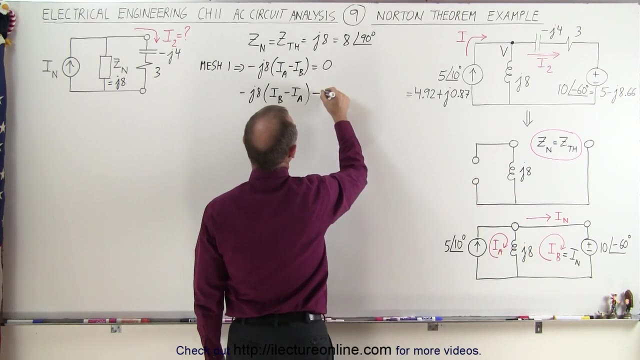 so in that case we have minus j8 times. but in this case we go in the same direction as ib. so we go ib minus ia. we come around here, nothing up here, and here we drop across this voltage. that's going to be minus 10, with a phase angle of minus 60 degrees, and that adds up to zero. so it's. 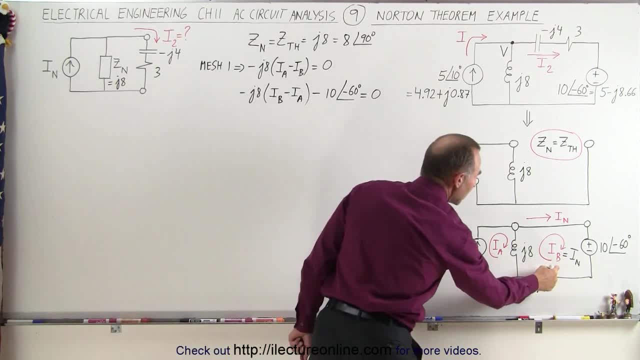 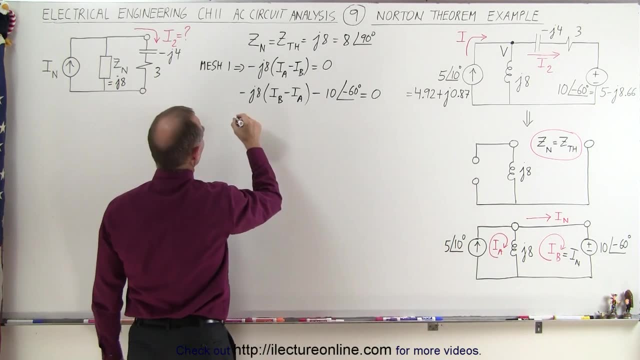 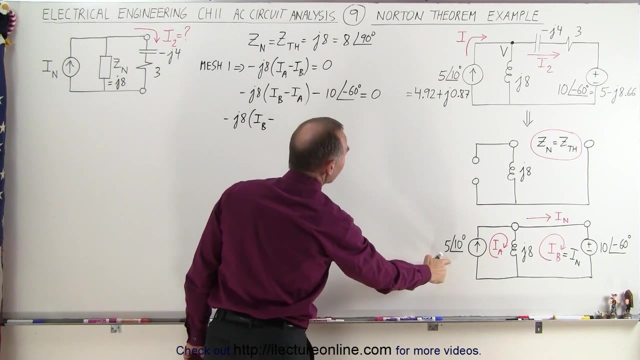 still nice, really simple equation. since we're looking for ib and we know that ia is going to be equal to the source current, right here. we can then replace it by the source current. so now we have minus j8 times ib, minus the source current. now, instead of writing it like this, let's see here: 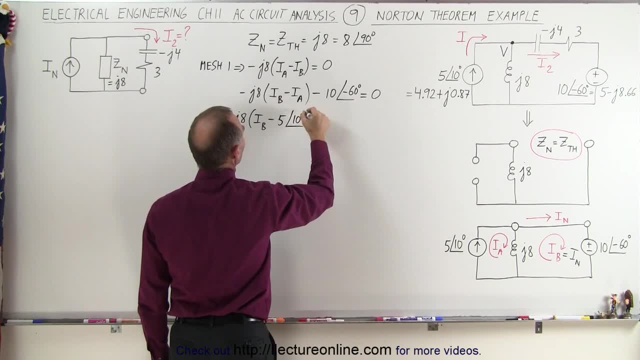 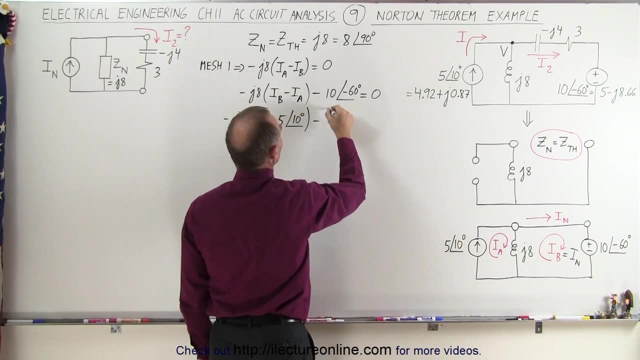 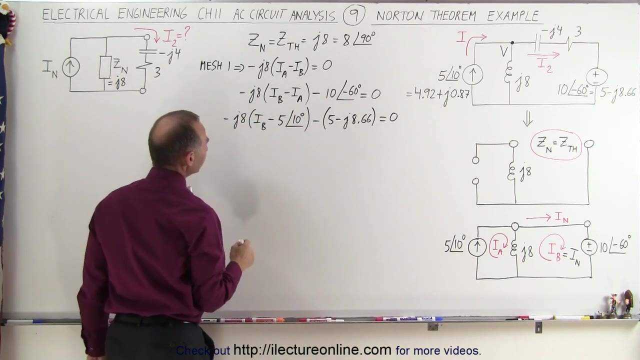 uh, no, we'll. we'll go ahead and write like this. so with minus five, with a phase angle of 10 degrees minus, To subtract this from this, I'm going to change this into minus 5. minus J8.66 equals 0. Multiplying this so we have minus J8 times IB. 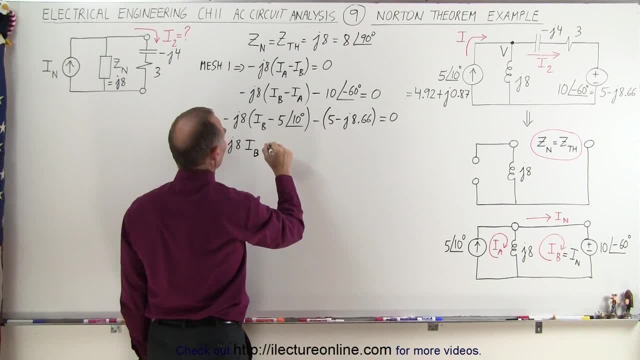 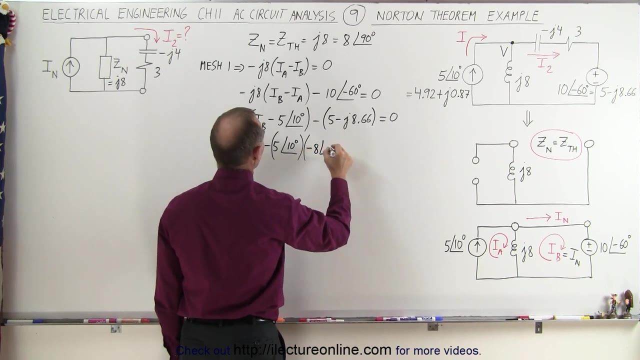 There we go Now this. multiplied times this, we have minus 5 times the phase angle of 10 degrees. And multiplying that times minus J8, that would be a minus 8 with a phase angle of 90 degrees. Let's see if I got the minus signs correct. 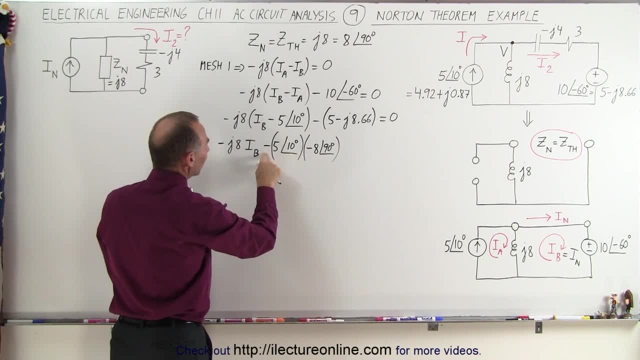 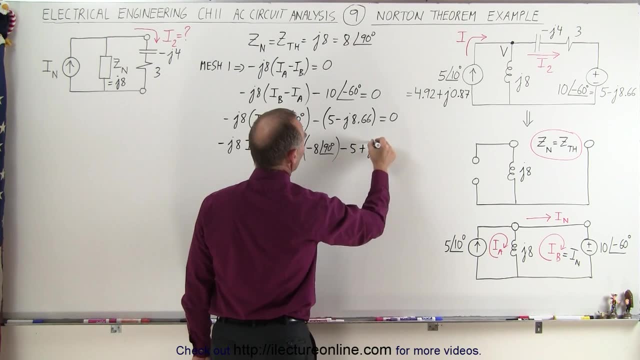 So I have a minus here, times a minus here. That gives me minus times minus, which is plus 5 times 8.. Yep, that looks good. And then here I'm going to say: minus 5 and plus J8.66 equals 0.. 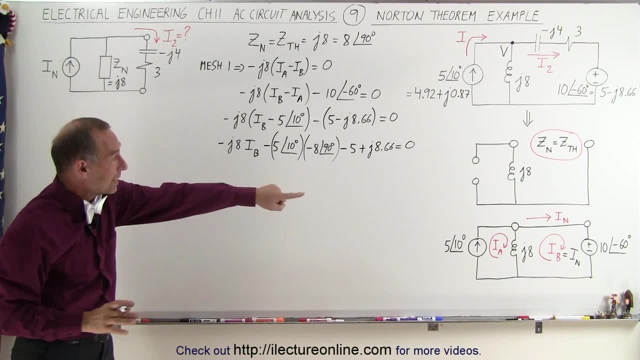 Okay, so remember that, ISB. what we're trying to do is we're going to subtract this from this. What we're going to do is going to be the Thevenin or not the Thevenin, but the Norton current. 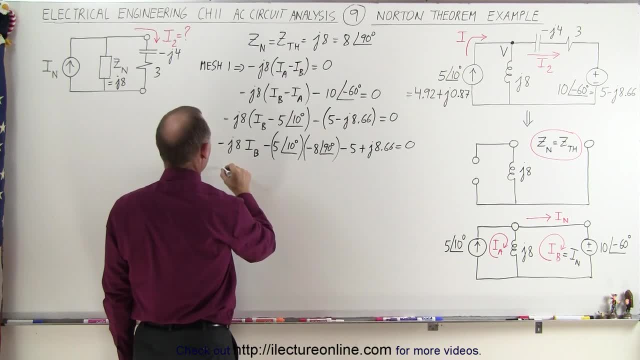 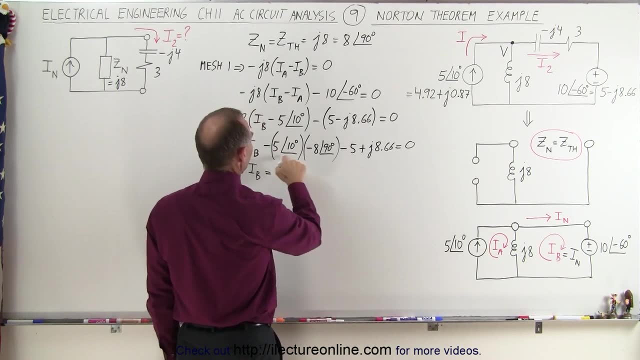 Okay, so let's multiply this out. So now that gives us minus J8. ISB is equal to this times this. Oh no, no, we'll wait for that Next step. So I'm going to multiply this out. so this is going to be plus 40, with a phase angle of 100 degrees. 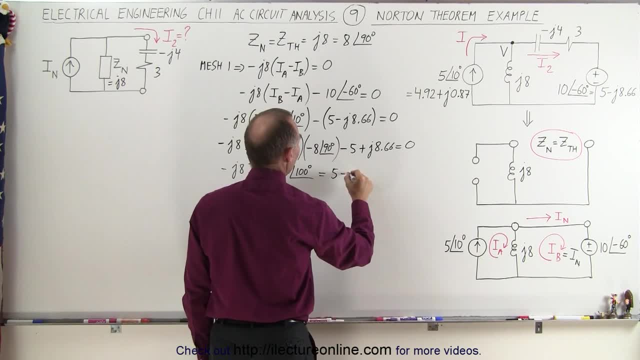 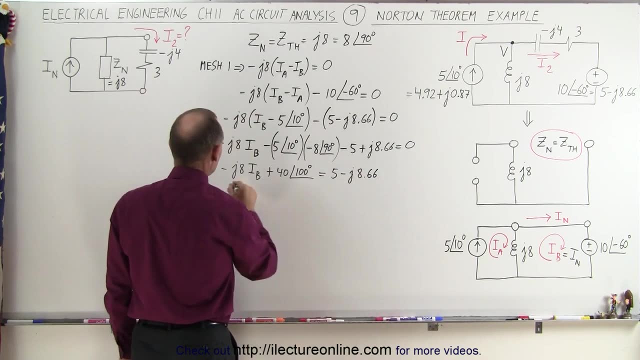 And moving this over. so this is going to be equal to 0.. So this is going to be equal to a positive 5 minus J8.66.. And then move this across. Before we do that, let's do the next. 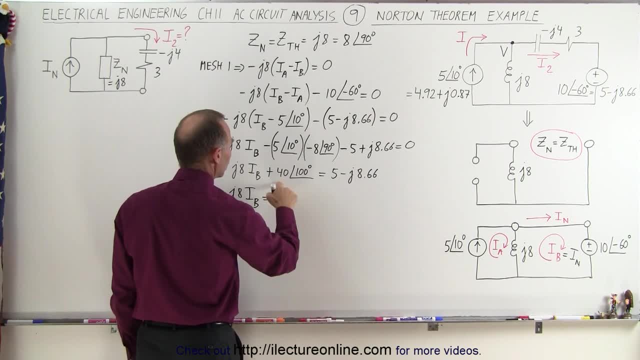 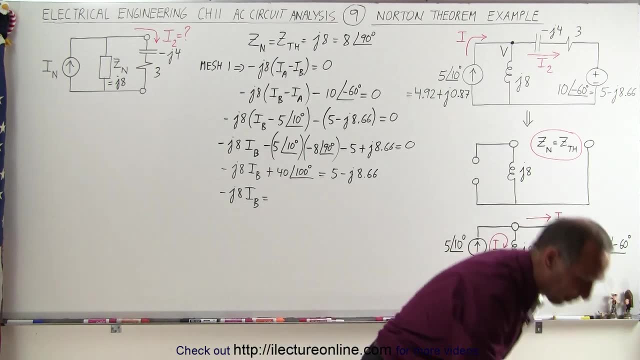 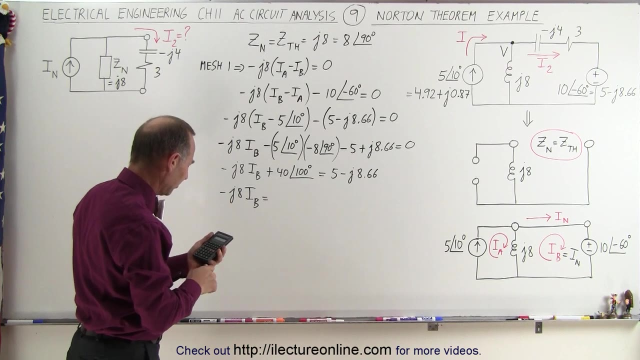 So minus J8, ISB is equal to this Almost. have that memorized by heart. but there's my calculator. Couldn't find my calculator. Okay, so 100 degrees. Take the cosine of that times 40, which is minus 6.95.. 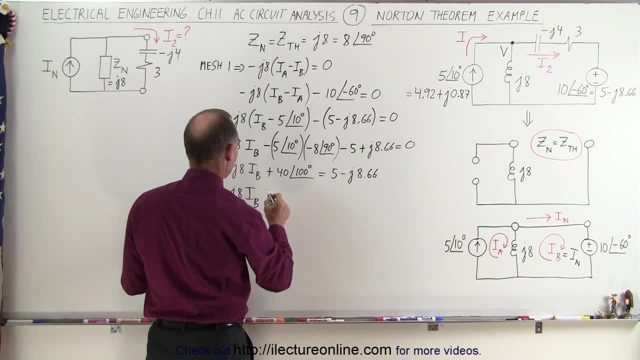 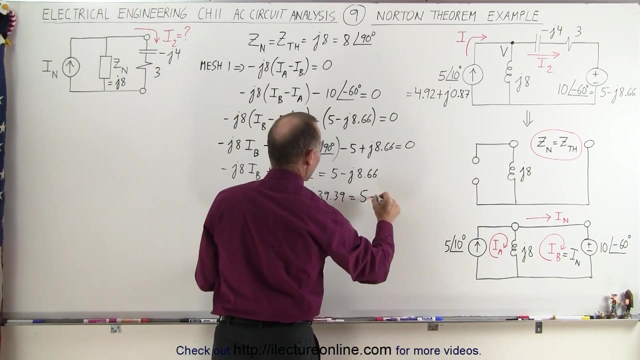 Okay, So we're not going to subtract yet. So we have minus 6.95 for the real part, and that would be plus J and that would be 39.39.. Now, remember that one That's equal to 5 minus J8.66.. 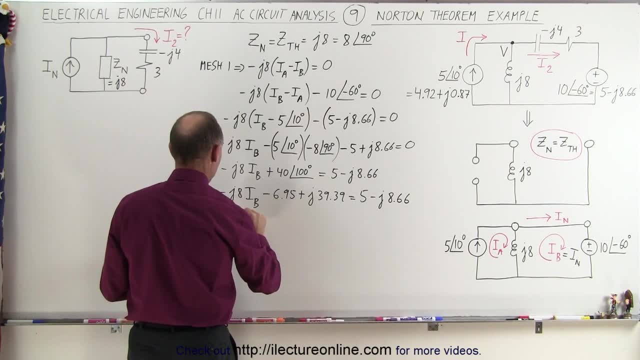 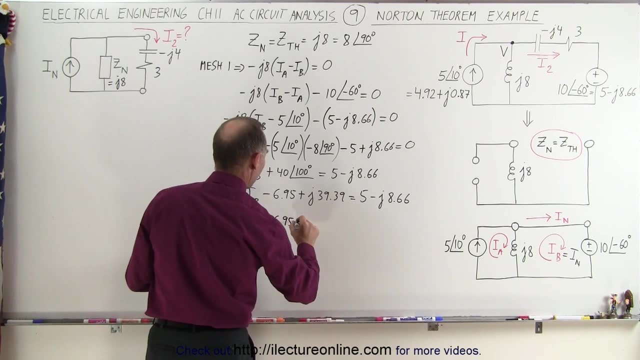 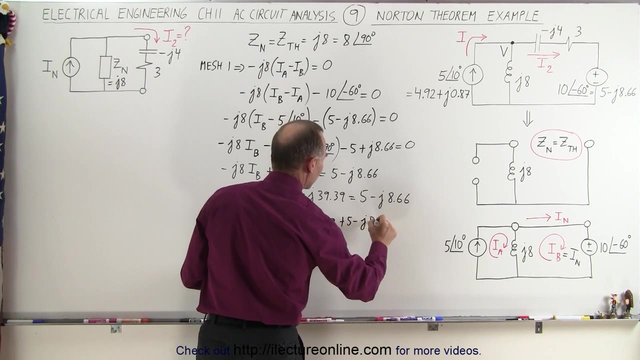 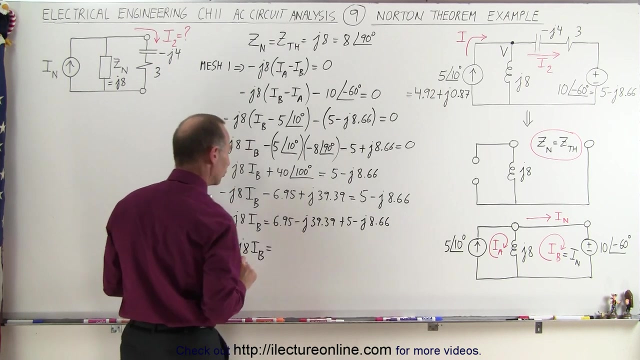 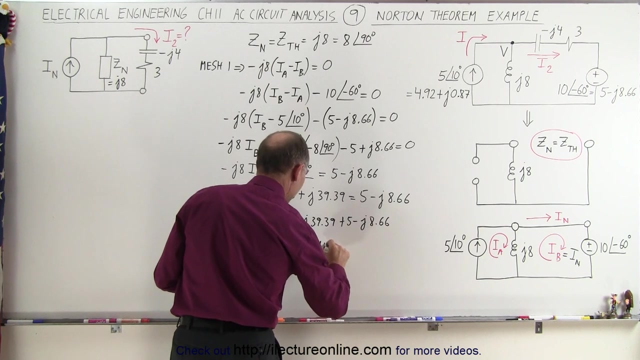 Now, moving this across the other side, we have minus J8 times ISB is equal to. that's a positive 6.95.. That's equal to 5 minus J39.39 plus 5 minus J8.66.. If we now combine that, we get minus J8, ISB is equal to 11.95 minus J, that would be 48.05.. 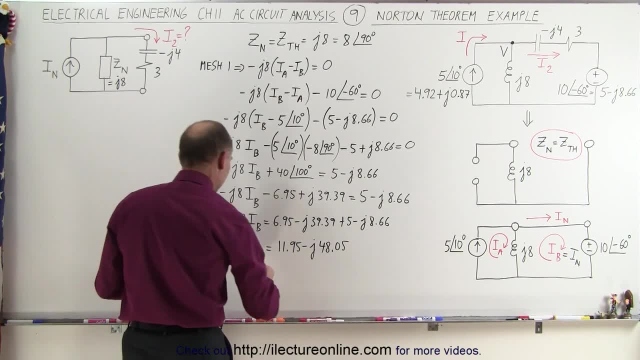 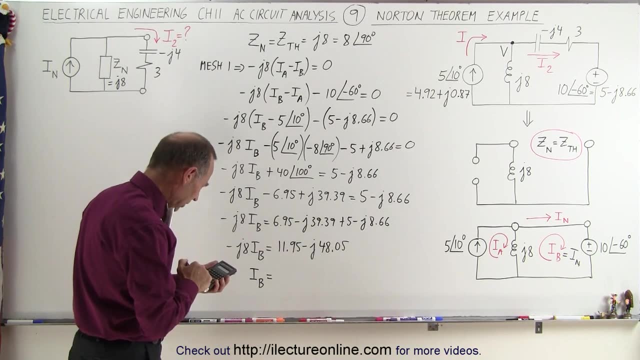 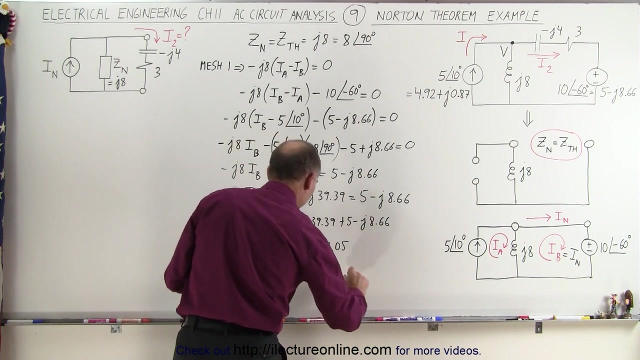 And then we have ISB is equal to: when you combine this, we have 11.95 squared at plus 48.05 squared equals. take the square root, that's 49.51, 49.51, with a phase angle of 48.05 divided by 11.95.. 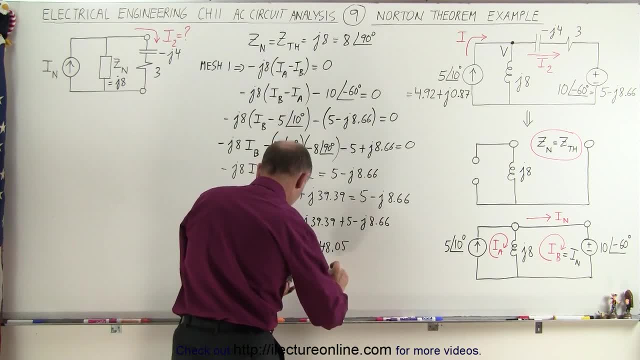 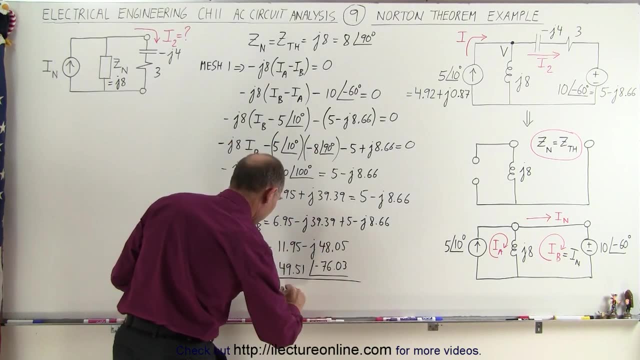 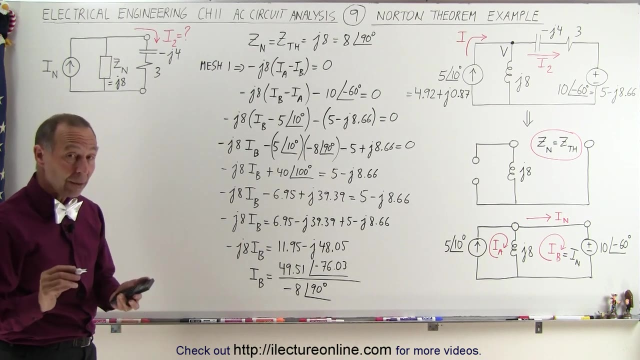 Take the inverse tangent, that would be a minus 76.03.. And we're going to divide that by when we bring this over here, that would be a minus 8, with a phase angle of 90 degrees. Okay, so now we can go ahead and divide one by the other. 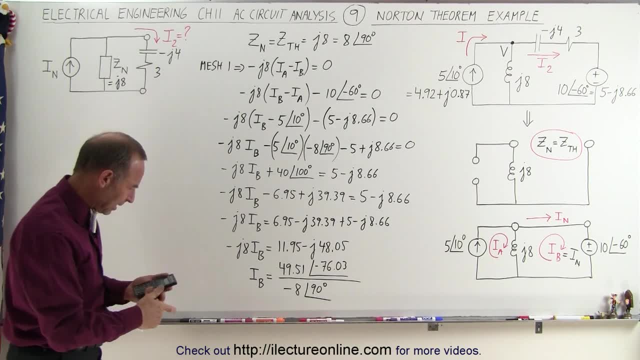 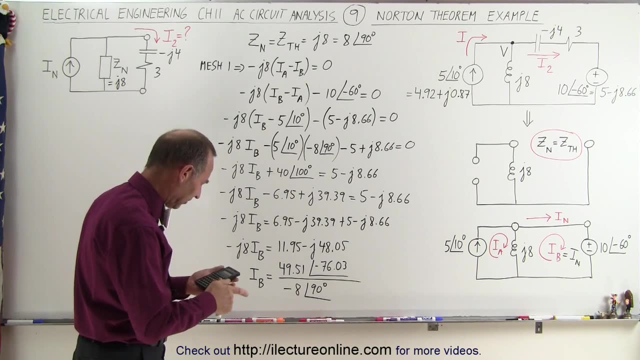 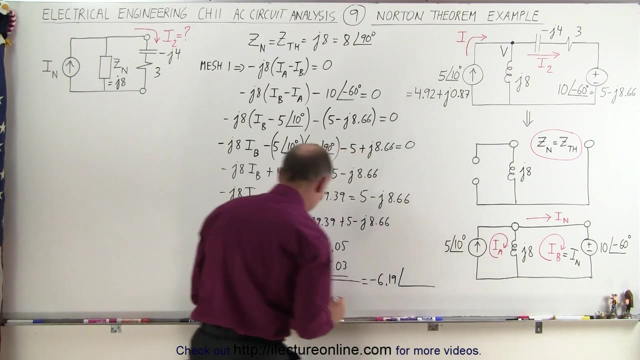 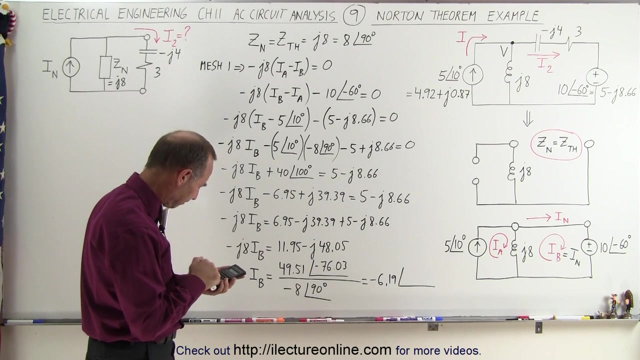 We have 49.51 divided by 8.. That's whoa. let me try this again: 49.51 divided by 8 equals- yes, that's a 6.19.. So minus 6.19.. So minus 6.19, with a phase angle of 76.03, 76.03, minus 90. 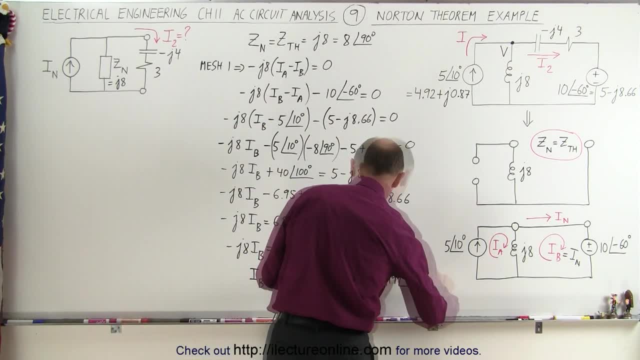 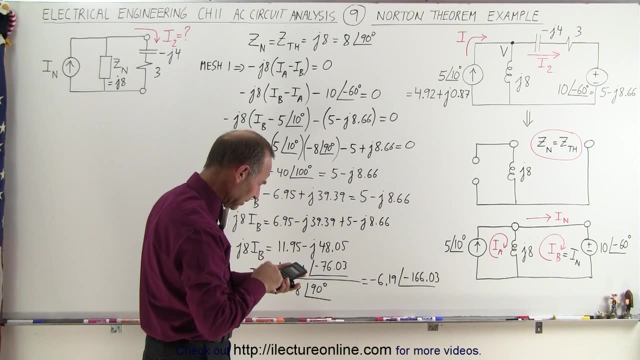 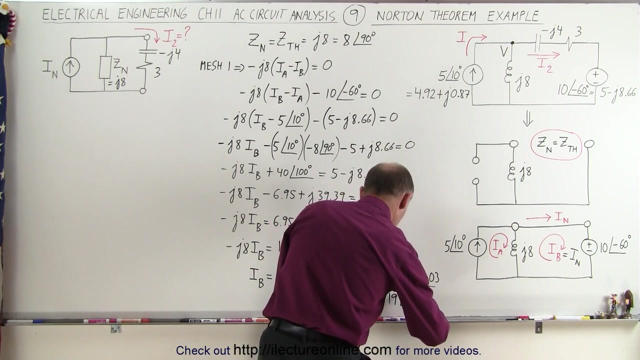 That's a minus 166.03.. And then if we take this and turn it into a positive, we're going to add 180 to that, So we end up with whoa 166.03.. 180 is that would be equal to a positive 6.19, with a phase angle of 13.97 degrees, of course. 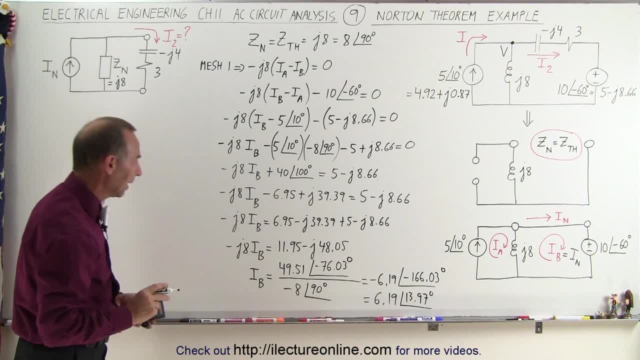 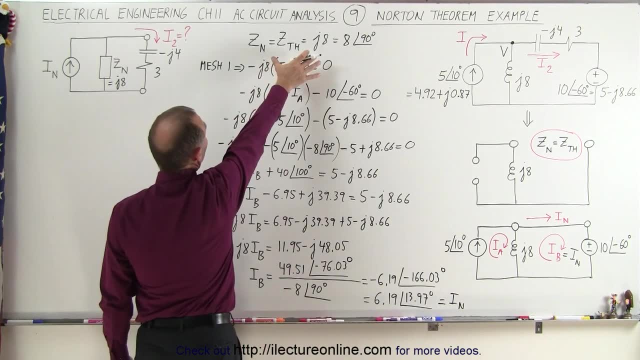 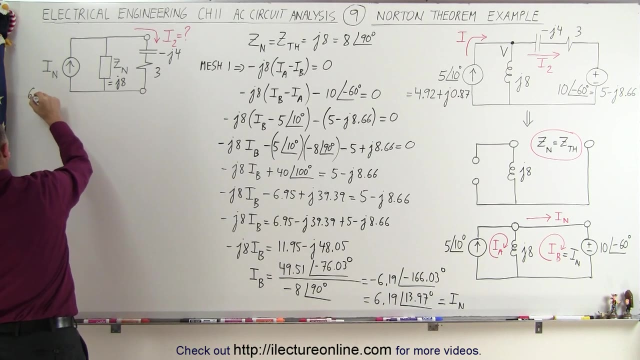 this is degrees, and degrees can't forget the degrees there. that's, of course, equal to our Norton current. so now that we have our Norton impedance and we have a Norton current, we can plug that in here. so this is going to be equal to 6.19 with a phase angle of 13.97 degrees. 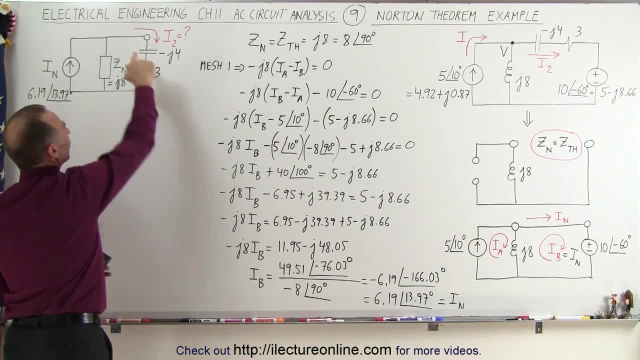 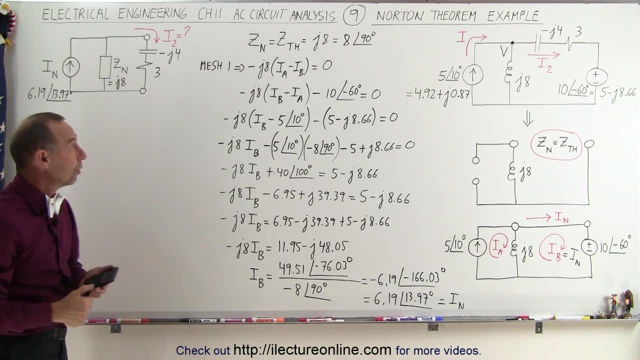 and the impedance we have as well. now, how do we find I2? how do we find the current? through our load impedance, the capacitor and the resistor? well, we're going to use what we call a current divider. we can say that I sub 2 is equal to the. 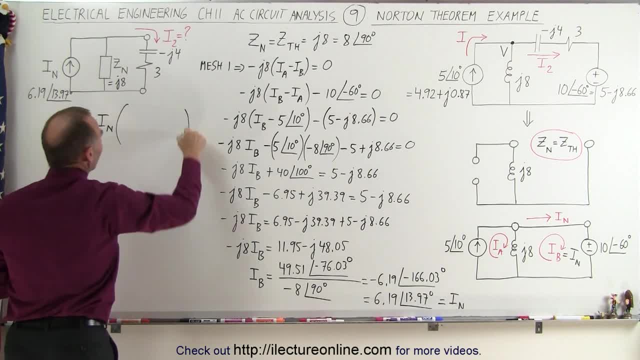 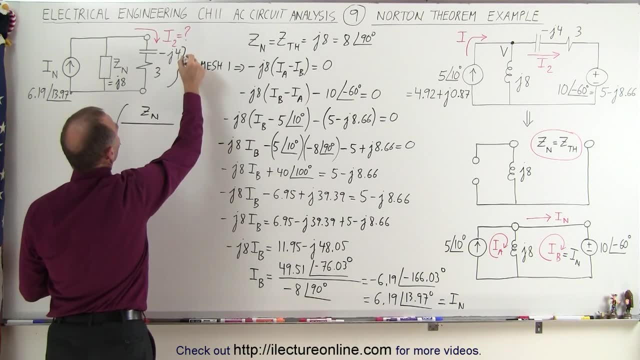 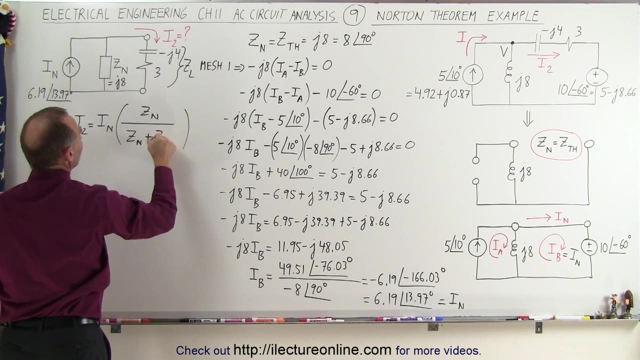 source current I sub N times the impedance in the other branch, which is Z sub N, divided by- and I'm going to take these two combined and this is going to be what we call the load impedance- divided by the sum of the two impedances, Z sub N plus the load impedance. so in this case this is equal to 6.19. 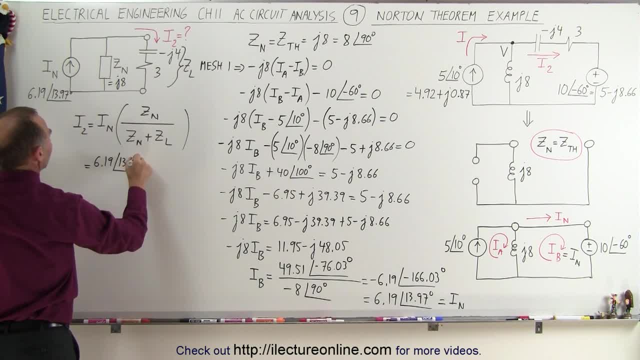 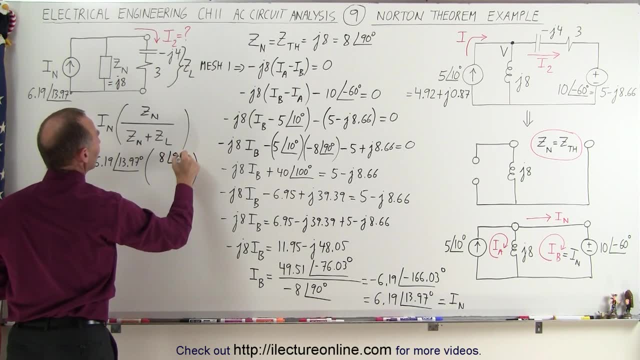 with a phase angle of 13.97 degrees, multiplied times the Norton current I sub N, times the impedance in the other branch, which is Z sub N, divided by Norton impedance, the Norton impedance which is going to be 8, with a phase angle of 90 degrees. 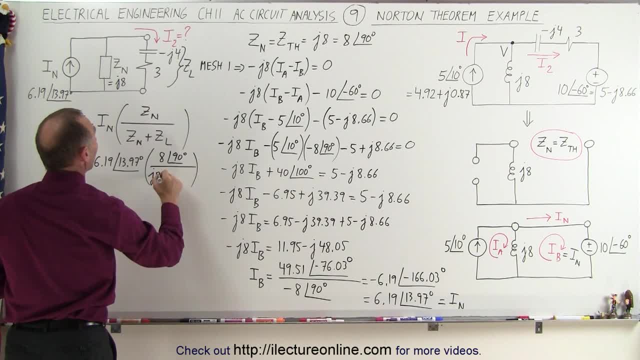 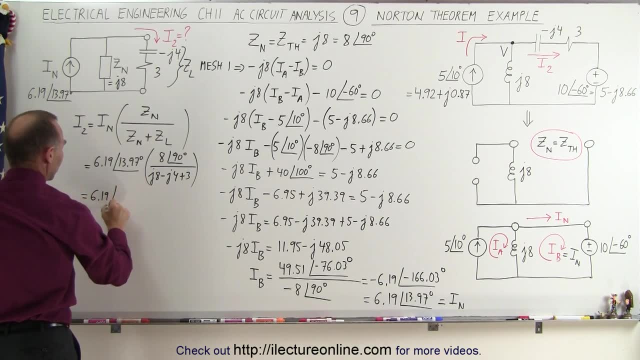 divided by in the denominator, we got J8 minus J4 plus 3. this is equal to 6.19, with a phase angle of 13.97 degrees. multiplied times eight, with a phase angle of 90 degrees, this is going to become 3 plus J4, which simplifies to 5, with a phase angle of 53.6,. 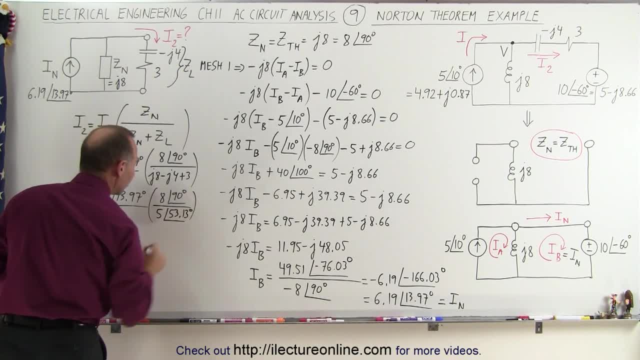 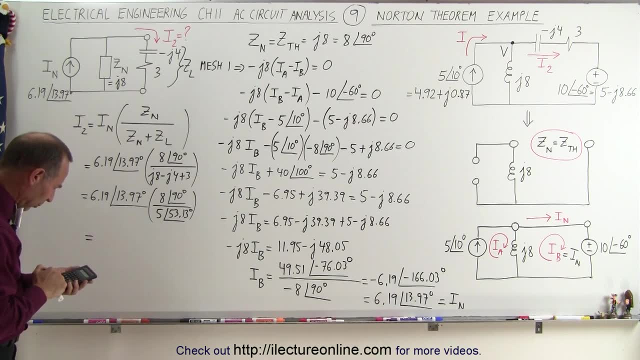 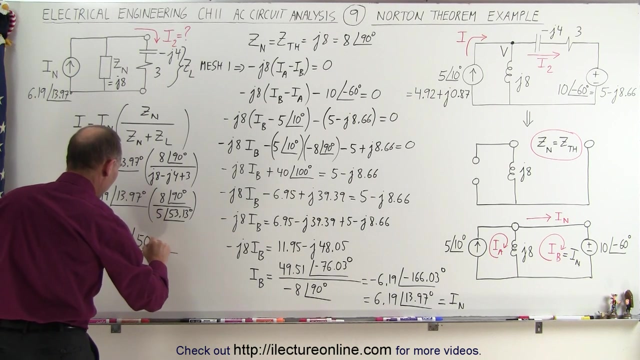 with a phase angle of 53.13 degrees. and now we can work all this out, and so this gives us 6.19 times 8, divided by 5, which is 9.90. with a phase angle of 13.97 plus 90 minus 53.13, that gives us a phase angle of 50.84 degrees. 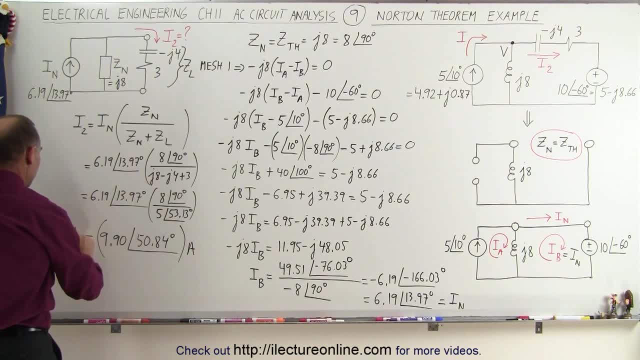 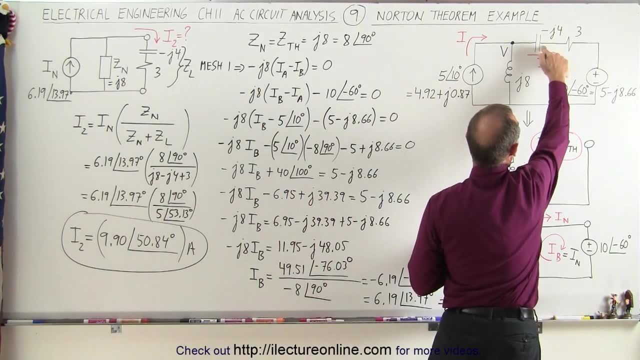 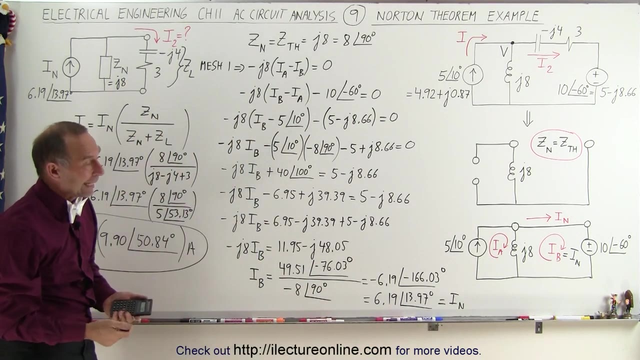 of course this is in terms of amps, and this would then be i sub 2, which is the current, through the branch we're looking for the capacitor and the resistor up in there, that circuit. so there's our sixth method. it's called the Norton theorem method. I don't like. 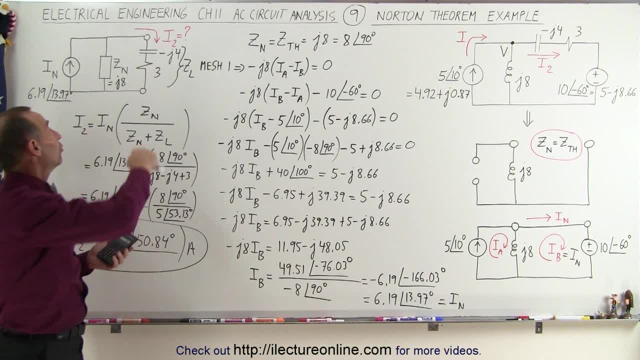 it quite as much as I like the Thevenin method, because Thevenin method uses the series circuit, here equivalent circuit. the Norton of course uses a parallel and maybe a little bit more complicated to figure that out. also it's a little bit more work trying to find the current to the short here. 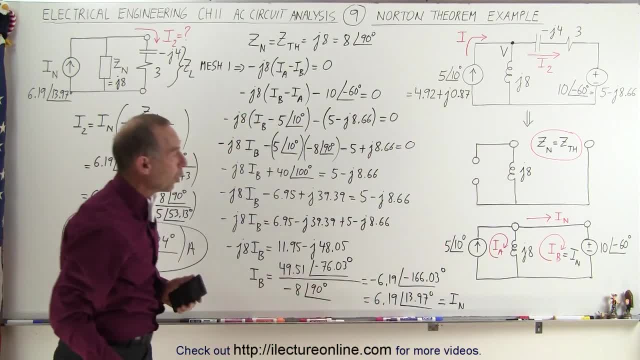 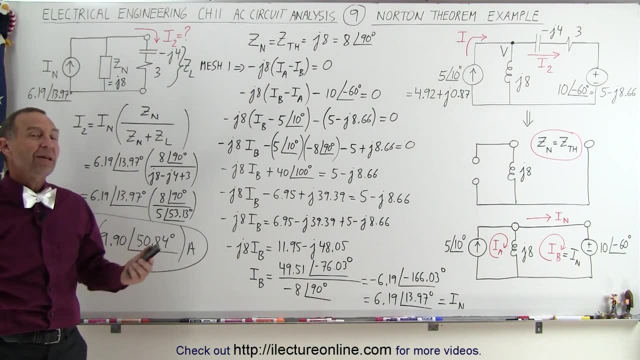 between the two terminals when the short replaces the load impedance. but it's a very valid method and in some cases it's also one of the easier methods to use. so now you may say we've seen six different methods to solve the same circuit. which method should you use? the one you like the best. 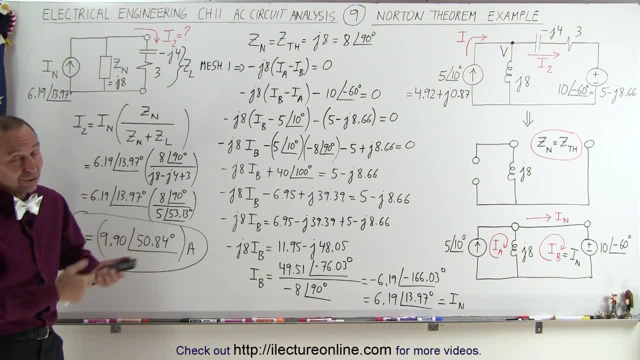 or the one you're told to use. sometimes you have no choice. they say: use this method for that circuit. one thing you could do if you're taking a test and you're supposed to use a particular method and you get an answer. you're not sure if it's right, but you can see that, think, oh, maybe I can. 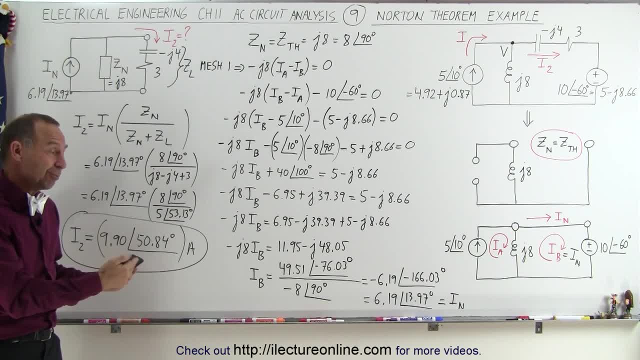 use a second method, and if you get the exact same answer with a second method, then you're going to. then you probably were correct, and that's kind of nice to do so: six different ways solving the same circuit. now, of course, we're going to show you some additional examples of each different method. some